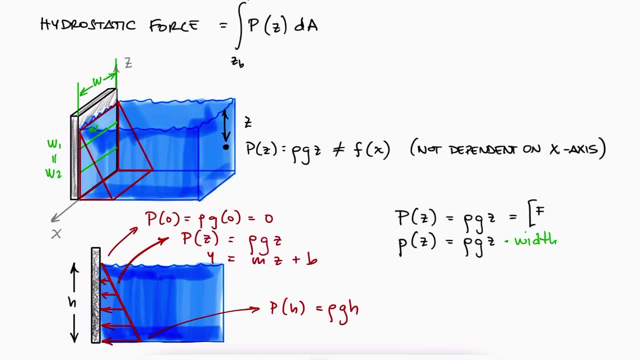 we would get new units for the pressure, which was once force over area, as force per length, which is consistent with the units of a typical distributed load. The integral from top to bottom of the distributed load, lowercase p times dc, would be the area of the horizontal axis. 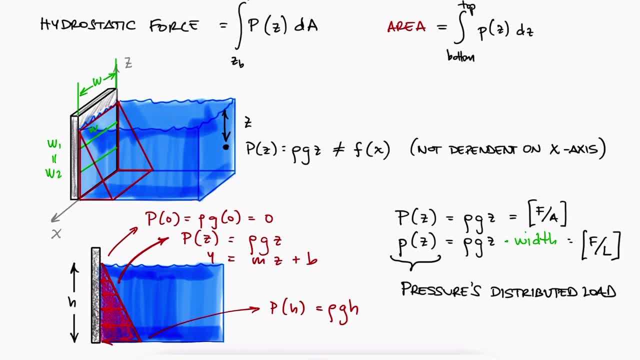 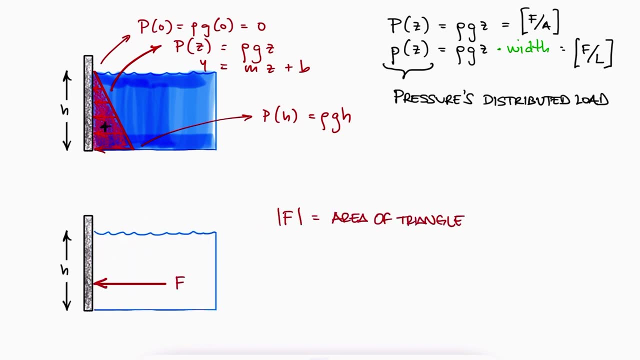 Under the curve of the triangle, just like it normally is for any of the triangular loads we studied in the previous video Link below to that specific section of that video And, just like any triangular load, the location of the equivalent point load with that magnitude is the centroid of 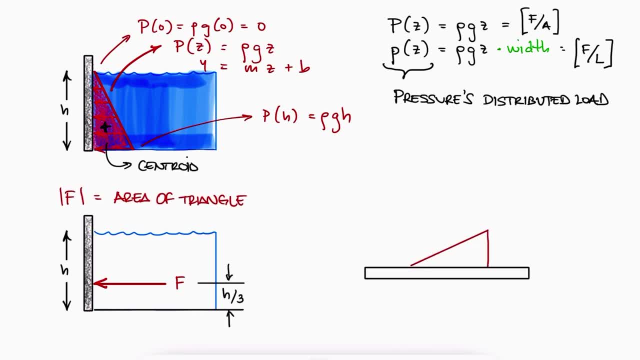 the triangle one-third from the base, As opposed to the triangular. loads on a beam, for example, we don't need to be given the highest value for the load density. In the case of a load on a beam, we would be given a Wx that reached something like 20 pounds per foot and that value referred. 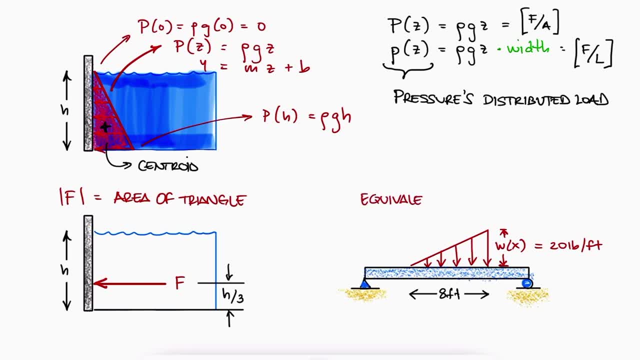 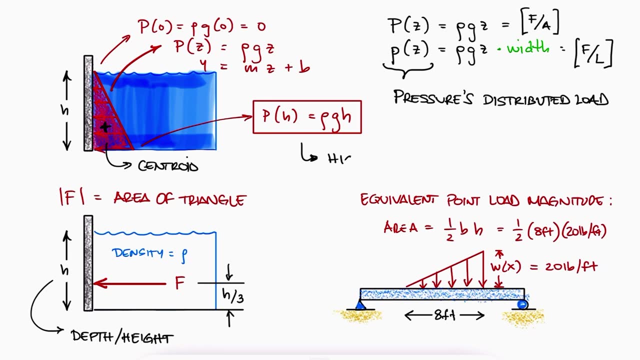 to that highest value, The area of the triangle would be one-half of the base, which is the length in the x-axis. times that 20 pound per foot height. In the case of hydrostatic pressure problems, by knowing the depth or height and the type of liquid we have, we can find that highest. 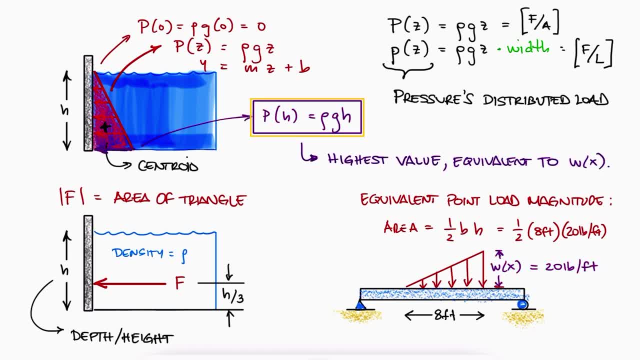 value from the distributed load, Since the pressure is rho- gh. by knowing the depth, we know h, and by knowing the liquid, for example water, we know rho- its density. The reason for calculating these hydrostatic pressure forces is to be able to calculate. 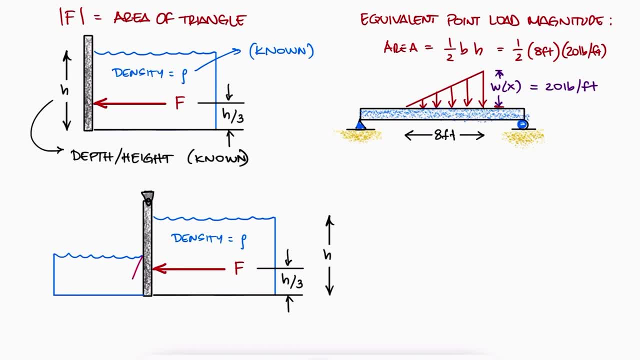 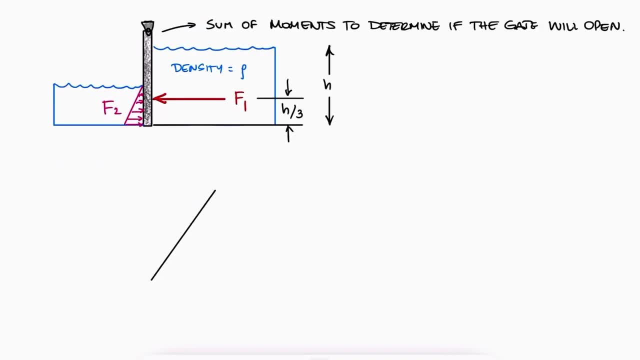 the reaction moment or forces that, for example, a gate has to generate to prevent the water from coming into the adjacent reservoir. Now the process of finding the resulting horizontal load from the fluid pressure doesn't only work for vertical surfaces in contact with a liquid. 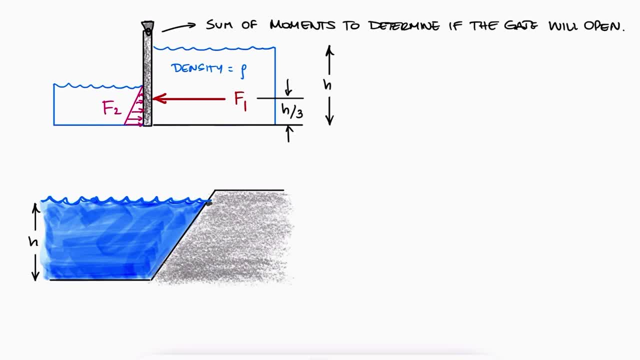 reservoir. If the surface is in contact with the liquid, it will be a liquid reservoir. If the surface is in contact with the liquid, it will be a liquid reservoir. If the surface is in contact with the liquid is inclined, the horizontal forces affecting the surface will be calculated in the 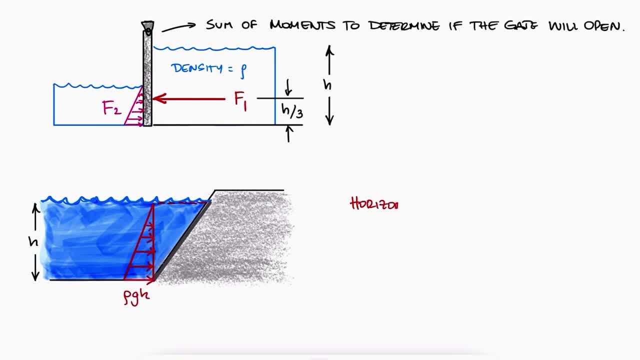 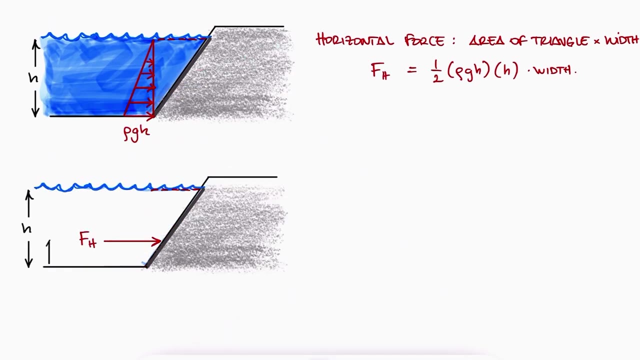 exact same manner, The magnitude of the equivalent point load in the horizontal direction would be equal to the area of the triangle, of the triangular distributed load, meaning rho gh times h divided by 2.. And just like before, it's also located one third of the way from the bottom to 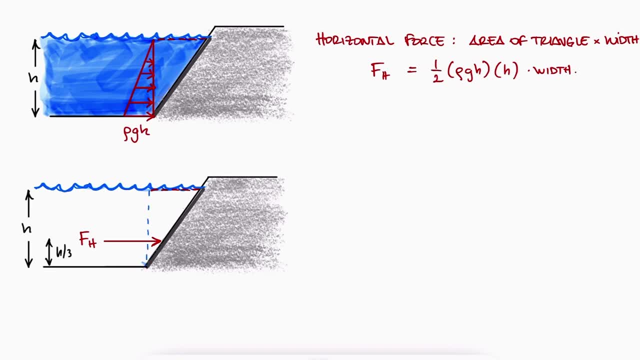 the top. Of course, on an inclined surface, the weight of the liquid above it, which is a vertical load, is the same as the weight of the liquid above it, which is a vertical load, which is a vertical load. In some cases, this weight will only be a triangle or the combination of a rectangle plus. 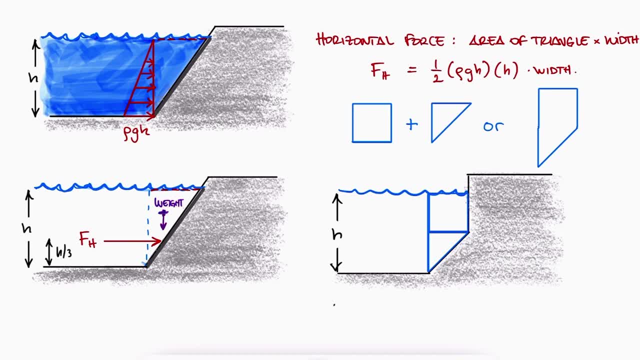 a triangle or just a trapezoid, The weight of the liquid would be the volume times the specific weight, which, for a 2D representation, is the area times the specific weight times the width. The location of the point load from the rectangular load is located right at the center. 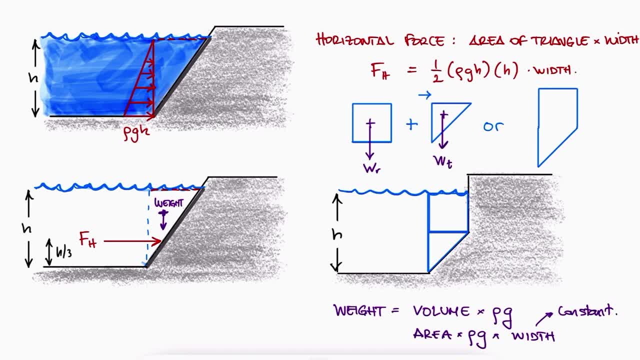 and again, just like with the pressure force, the location from the triangular weight is located one third of the way from the side of the triangle. Variation of these two situations: the vertical wall and the inclined one that begins right at the surface of the liquid. 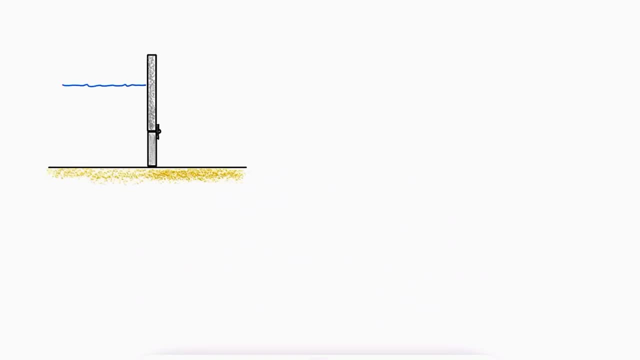 is if the walls or other member of interest is submerged beyond the surface of the liquid. For example, if there's a gate at the bottom of the reservoir and you can think of it as a valve that opens to drain a reservoir, the distributed load affecting the gate will 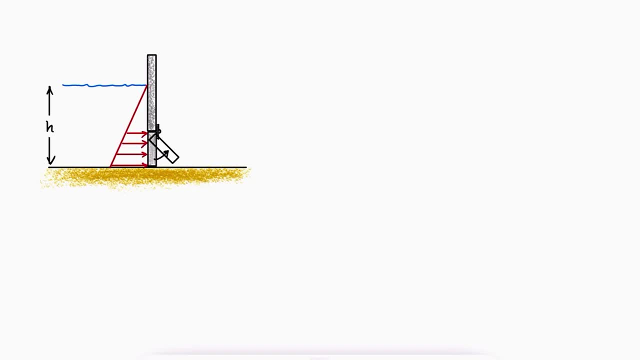 only be the portion of the hydrostatic pressure between the bottom and the top of the gate, which means the linear distributed load looks like a trapezoid And again, if you don't want to deal with the centroid of a trapezoid, to find the location. 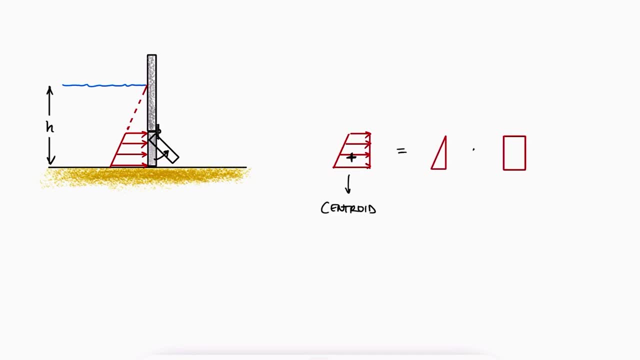 of the equivalent point load. you can divide it into a rectangle plus a triangle: The rectangle's point load located at the center of the gate's height and the triangle's point load located one third of the height of the gate from the bottom. 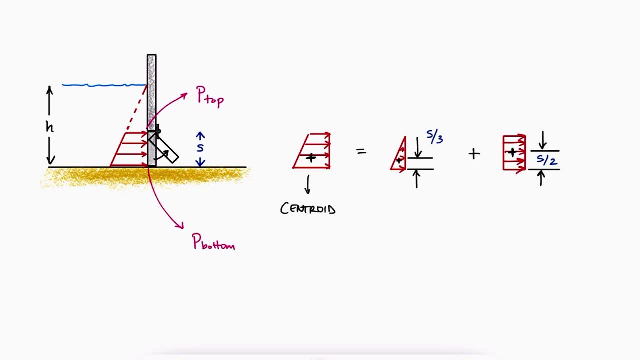 The value for the pressure at both the top and the bottom would just be rho g times z, where z is the depth or distance from the surface of the liquid. With these values, we could calculate the area of the rectangle as well as the area of the triangle. 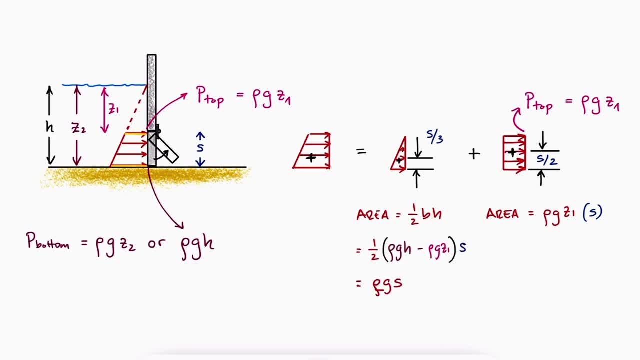 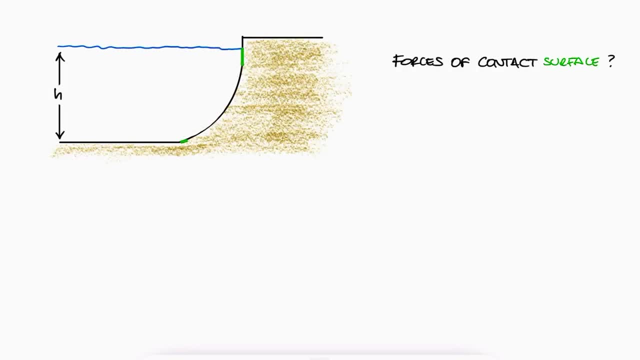 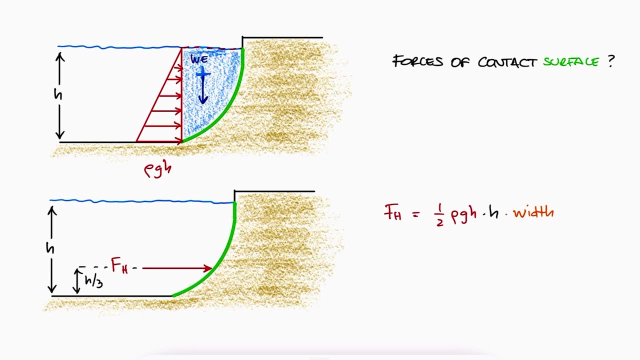 by finding the base as the difference between the distributed pressures. For any other shape of the floor of the reservoir, for example a curved bottom, the process would be the same: The pressure on the side is creating a horizontal force and the weight of the liquid above the curve is creating a vertical load. 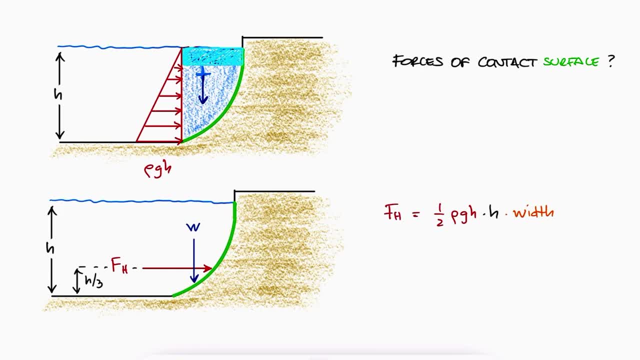 The weight is divided into one: a rectangle above the curve, just like we did with the flat inclined wall from before, and two, the weight of the remaining geometry, which can be calculated using everything we learned during the centroid and center of gravity. main video Link below if you haven't watched that yet. 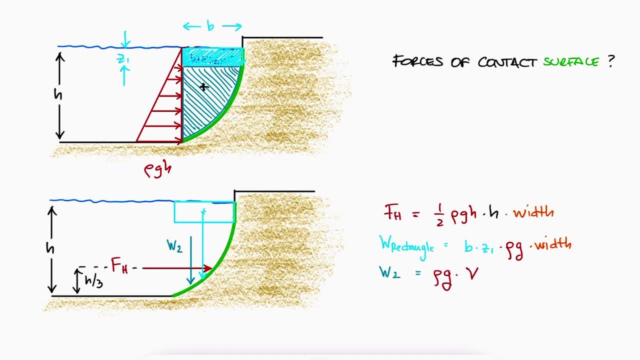 The equivalent force will be the specific gravity times the volume, which, in terms of the integral, is the width in the third dimension. we don't see times the area written as the integral about z of all the d areas along the z direction. This is usually written as a function of z. 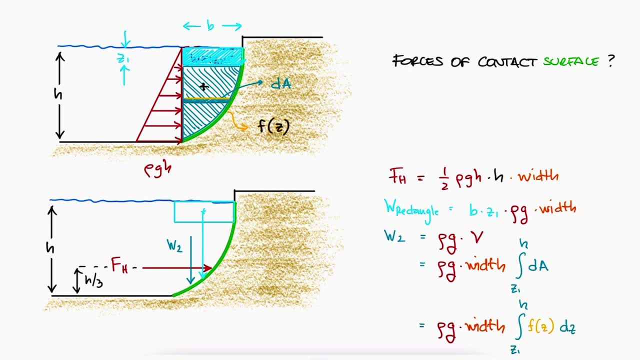 known due to the geometry of the floor slash wall, The location of the equivalent load would be at the centroid of the volume. again, link below to that portion of the video where we study center of gravity, center of mass or centroid of the volume for a shape described by a given math function. 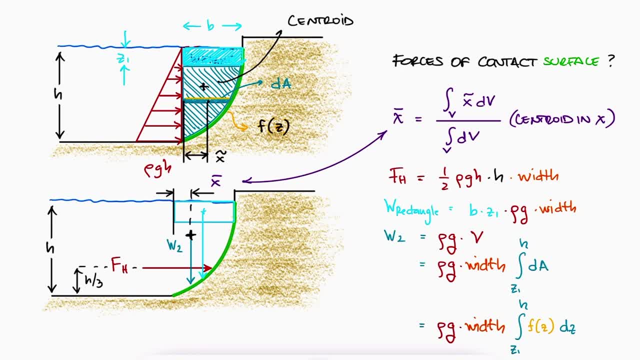 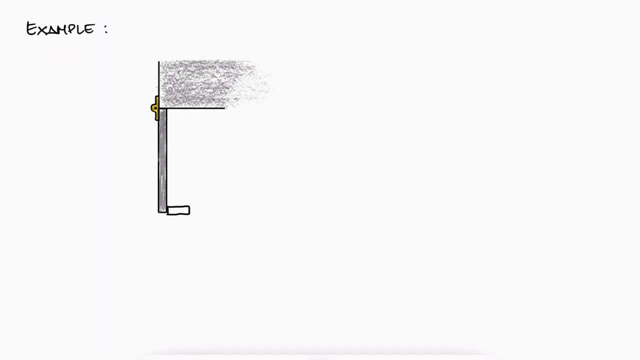 Let's take a look at a simple example where we make use of what we've learned today, And if you want to check out more complex problems, you can check out the 2 minute long video examples on this topic linked in the description below. 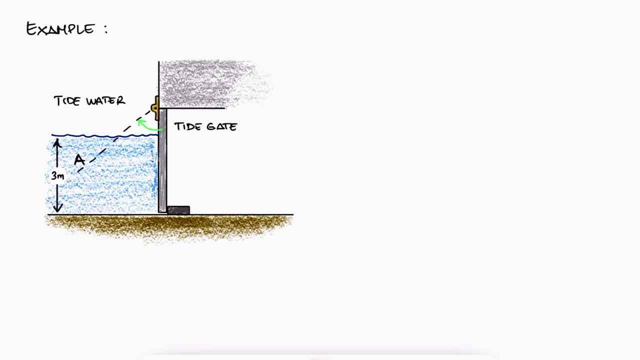 When the tide water A subsides, the tide gate automatically swings open to drain the marsh B. For this specific condition of high tide, shown what are the horizontal reactions developed at the hinge C and the stop block D. The width of the gate is 6 meters. 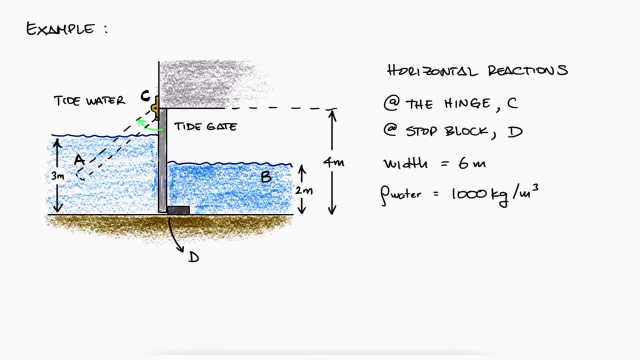 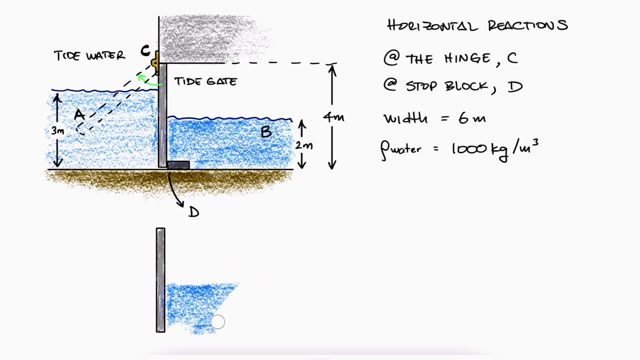 and the water density is 1000 kilograms per meter cubed. Remember to try to solve this problem on your own before watching this video. A free body diagram of the tide gate would show the reactions at C and D that we're looking for. 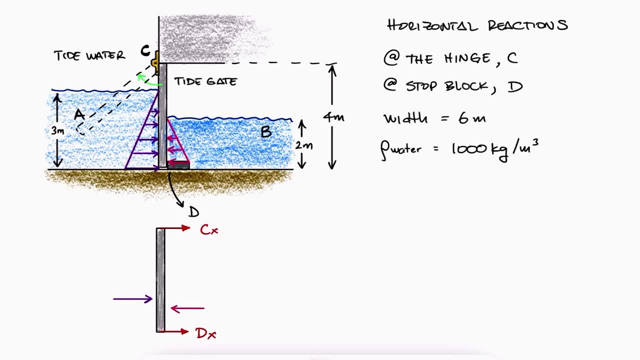 plus the two hydrostatic pressure forces, The maximum hydrostatic pressure on the left- let's call it E- would be equal to rho GZ, with the depth C being 3 meters. The hydrostatic pressure at point D would be that for a depth of 2 meters. 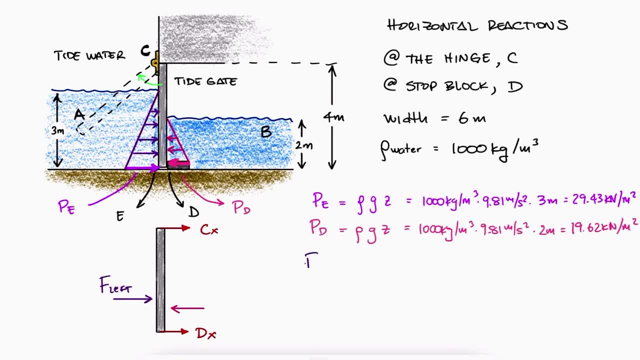 The force coming from the left side would be equal to the area of the purple triangle times the width of the gate. The force coming from the right side would be equal to the area of the pink rectangle times the width of the gate. The location of the purple force would be at the centroid of the left.